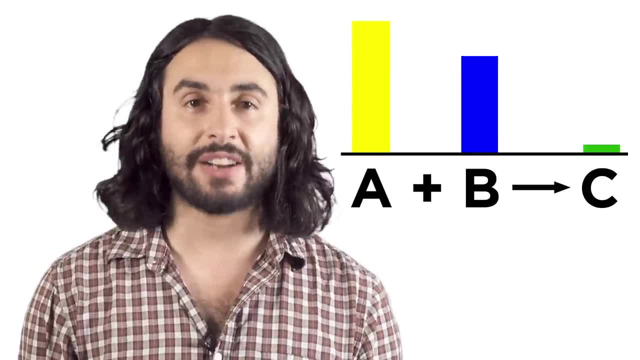 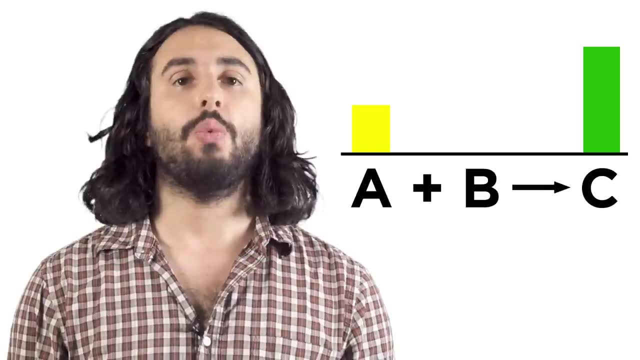 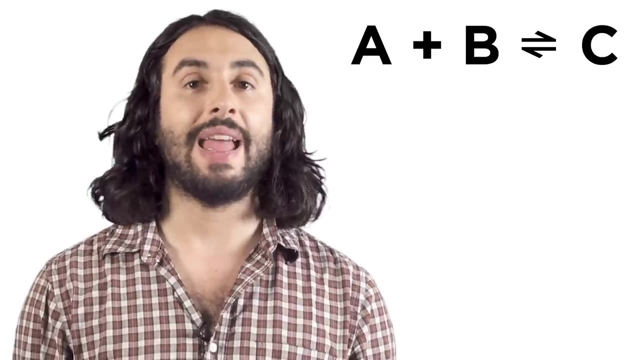 of the products to expect. but these were for unidirectional reactions, where we assume that all the reactants make products and then the reaction is over. with equilibria, it's a little more complicated to calculate what the consequences are. the concentrations of each substance will be at equilibrium, so we're going to 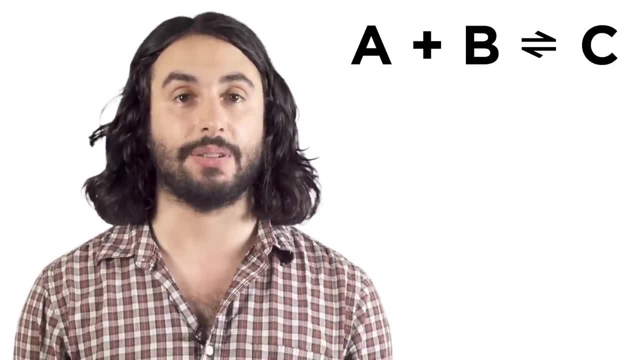 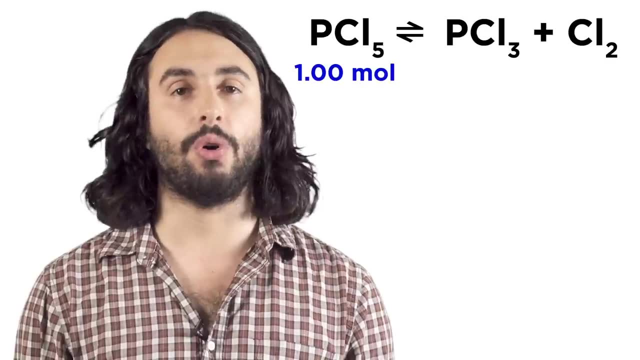 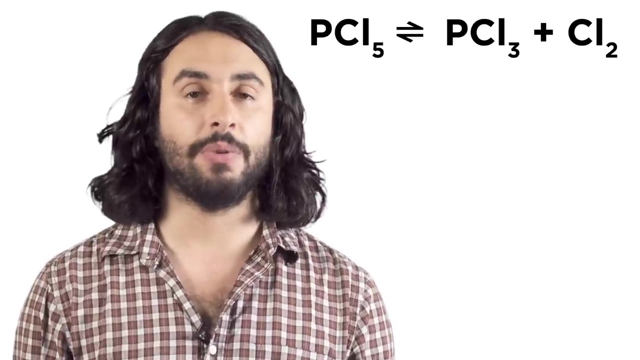 have to do a little bit of math to be able to describe the system. for example, let's look at this equilibrium. let's say we start with one mole of PCl5, allow the system to reach equilibrium and then, once at equilibrium, we measure that. 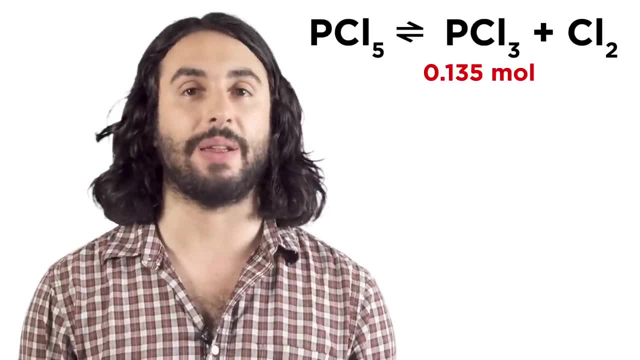 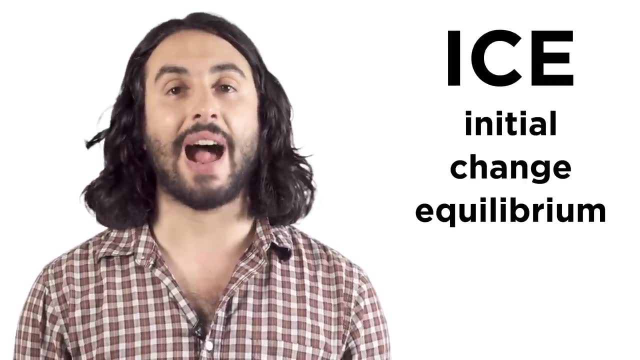 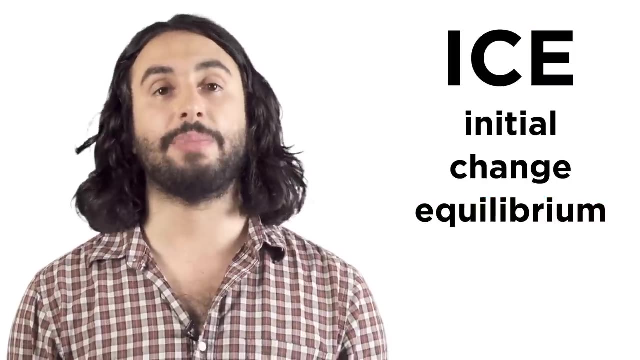 there are 0.135 moles of PCl3.. so how much of the other two things are there? to answer this, we can make something called an ICE box. these letters stand for initial change and equilibrium. we set them up like this. 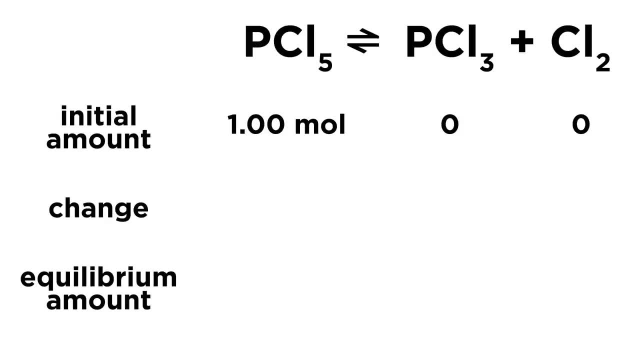 for initial: we put the initial amounts of each thing. we started with just one mole of reactant, so we put one there and zeros for the products, since there wasn't any of those at first. then for the change: we don't know exactly how much the change was to get to equilibrium. 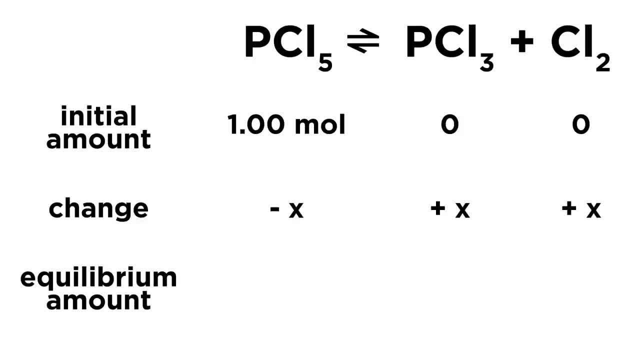 so we call it X for the reactant. we put negative X because it is being depleted and in this case all of the stoichiometric coefficients are one. so as X moles of reactant are being depleted, X moles of each product are. 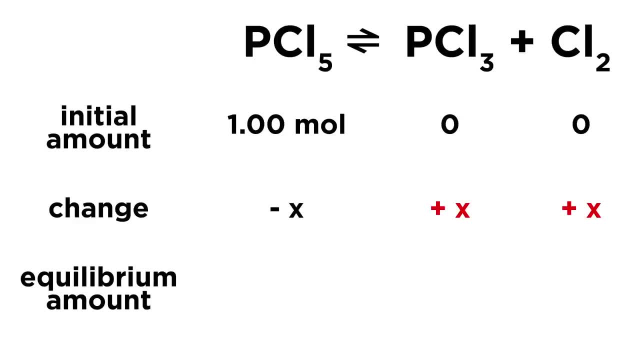 being formed. we would make these two or three X as necessary if the coefficients were different and for the products, X is positive because these are being formed. then, lastly, we add up the initial and the change to give the amounts present at equilibrium. 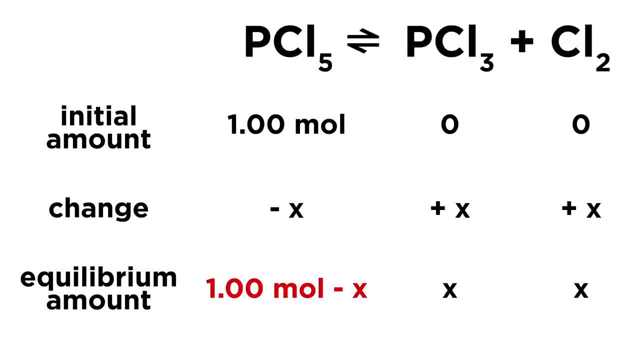 for the reactant this is one minus X, and for the products it's simply X. we measured the final concentration of PCl3 as 0.135 moles, which here will correspond to X, and we therefore know all the other concentrations by plugging. 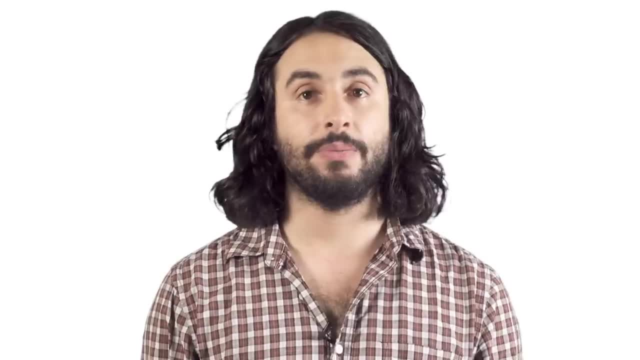 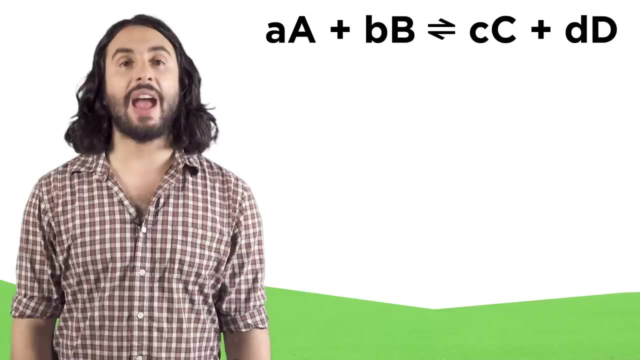 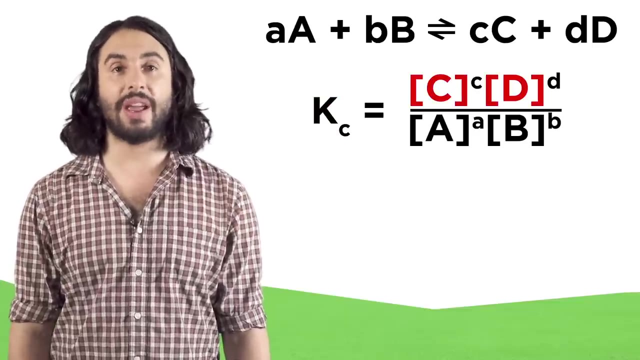 in X, simple. no well, it can get trickier, as we will see. but first let's learn about equilibrium expressions. every equilibrium has an equilibrium constant, Kc. it will be given by the concentrations of the products, each raised to the power of their stoichiometric coefficients over. 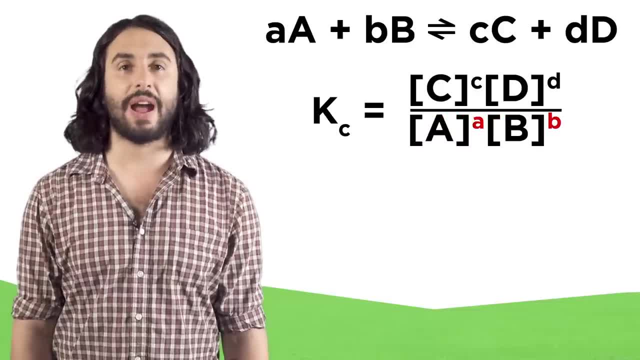 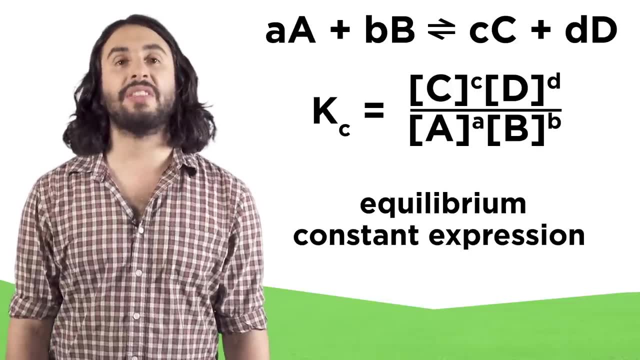 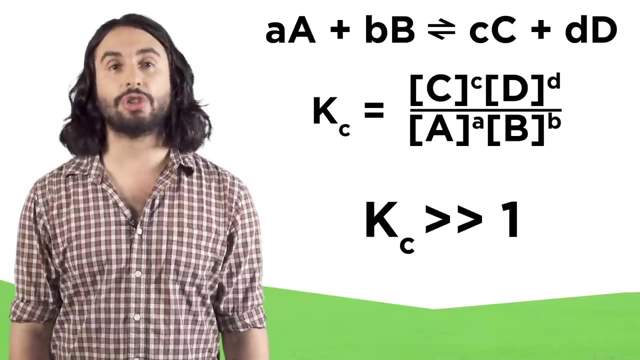 the concentration of the reactants, each raised to the power of their stoichiometric coefficients. this is called the equilibrium constant expression. one thing this constant tells us is whether the products or reactants are favored in the equilibrium. if Kc is much greater than one, that means the numerator is 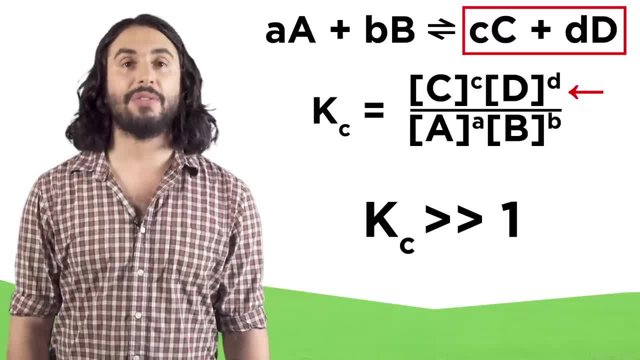 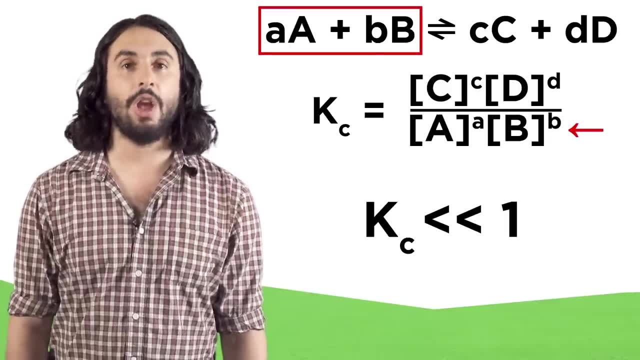 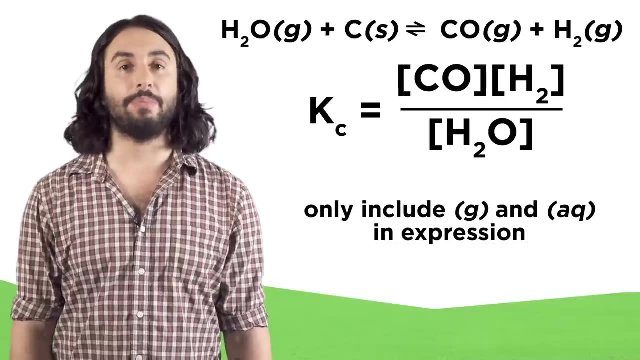 bigger, so we are creating more products. if Kc is much less than one, that means the denominator is bigger and we are creating more reactants. when we write this expression, we only take into account gases and aqueous species. solids and pure liquids will not be included in the expression, for example here. notice: 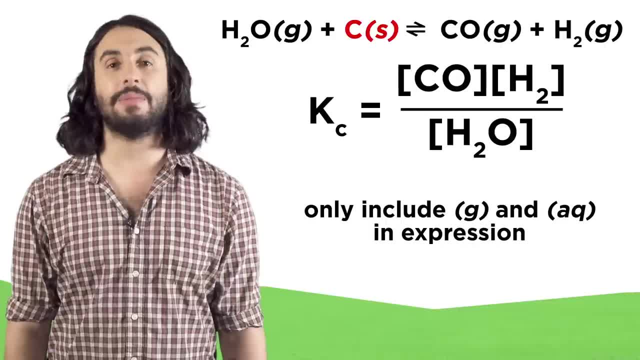 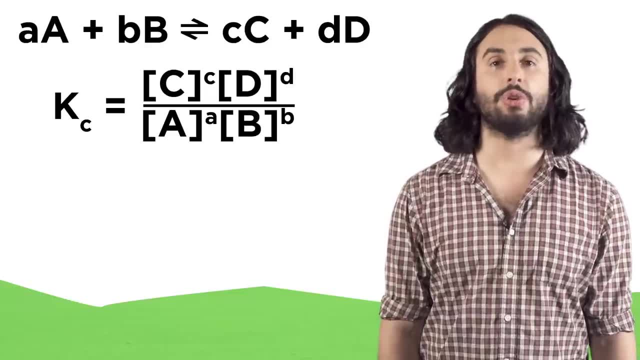 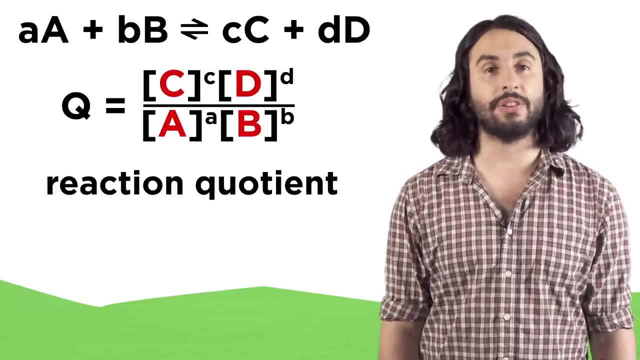 how carbon is not included in the expression, since it doesn't make sense to discuss a solid in terms of a concentration. sometimes we may want to predict which way a mixture will go given some non-equilibrium quantities. to do this, we plug the non-equilibrium values into the Kc expression to calculate the reaction. 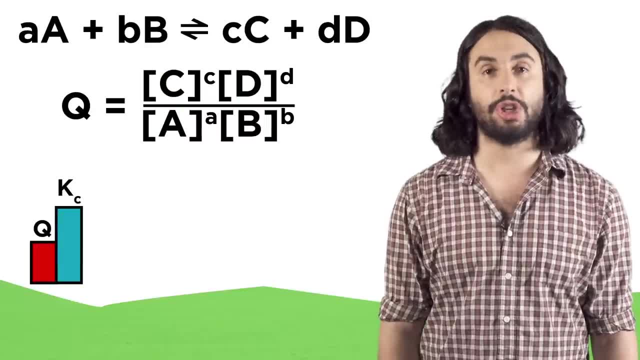 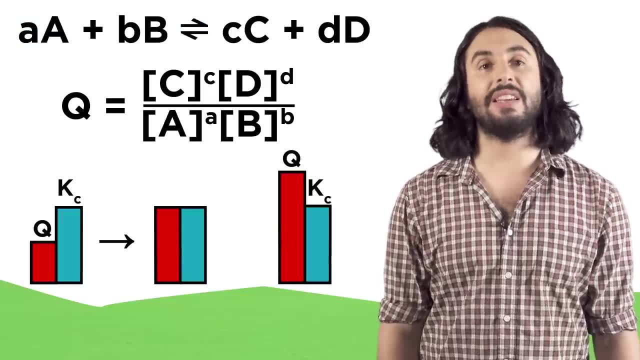 quotient Q. if Kc is bigger than Q, Q is more on the reactant side, so it'll make more products to equilibrate. if Kc is smaller than Q, Q is more on the products side, so it'll make more reactants. 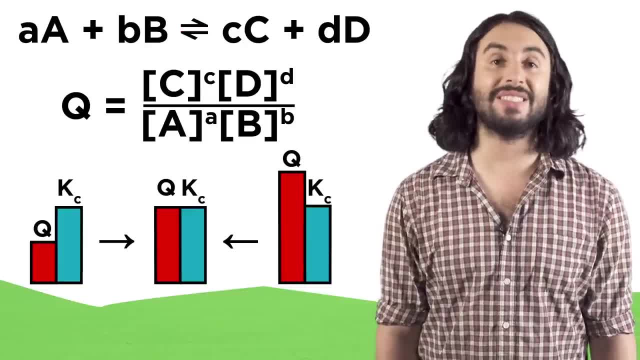 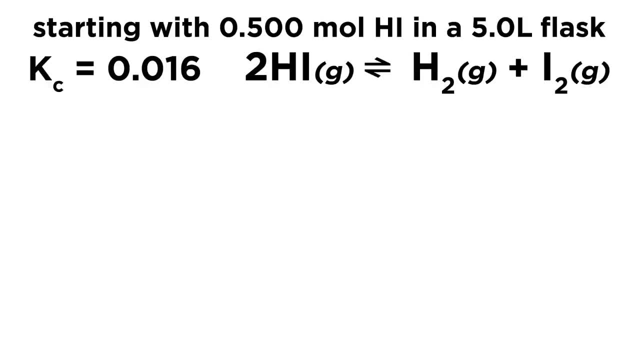 to equilibrate. when Kc equals Q, the system is at equilibrium. let's try a more difficult icebox. given the following information: calculate the equilibrium concentrations of each substance in terms of molarity. remember that molarity is moles per liter. so we set up our icebox and calculate the. 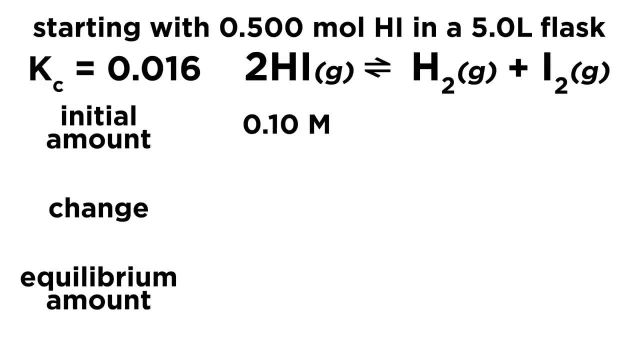 concentration of our reactant. that'll be the initial value and zero for the products. now here the change will be different for each substance because of the stoichiometry, for every two moles of reactant we get one mole of each product. so we have to subtract 2x here and add.